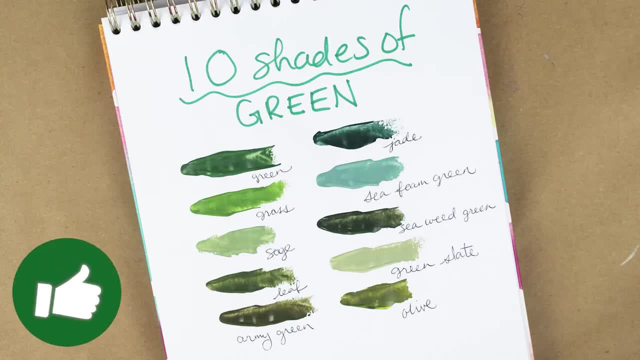 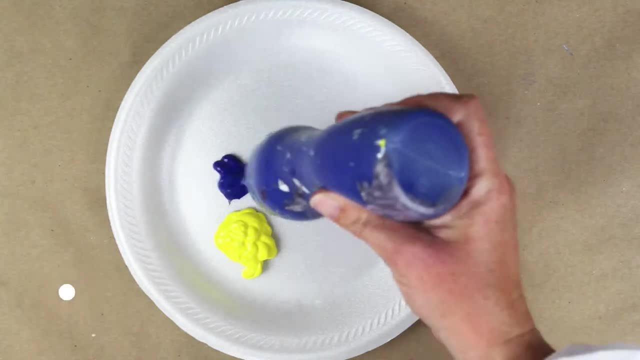 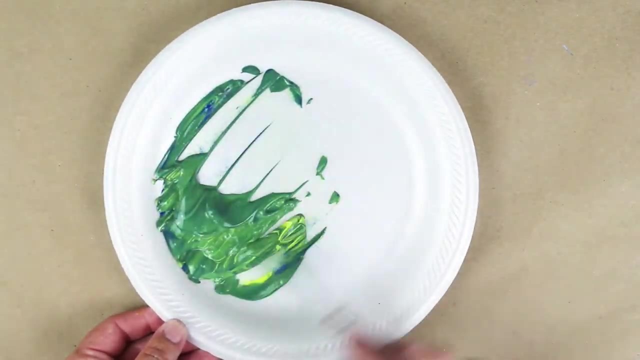 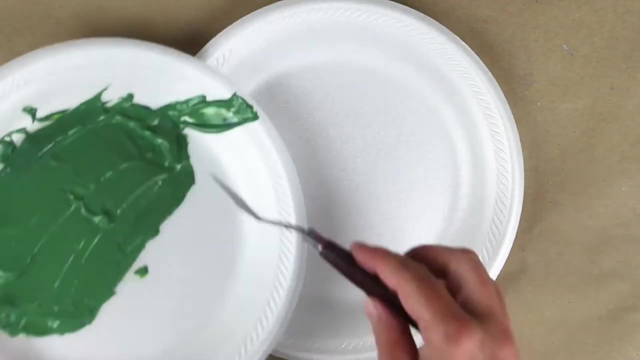 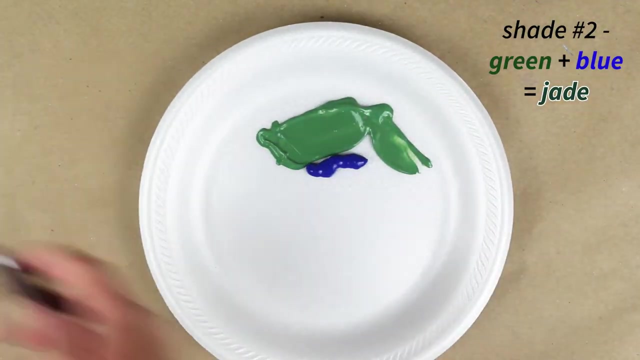 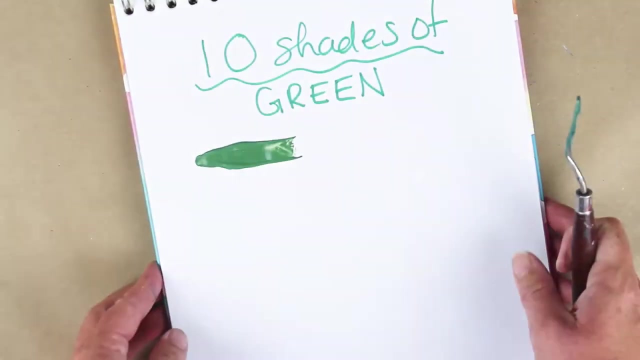 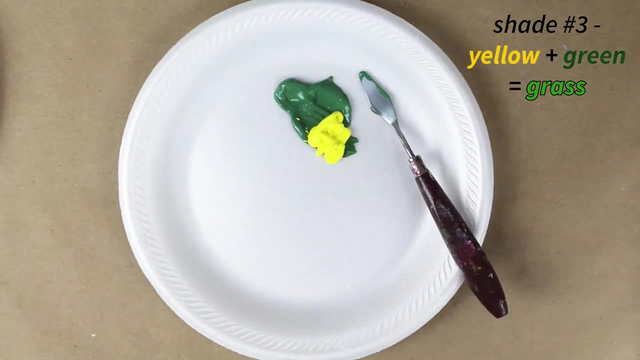 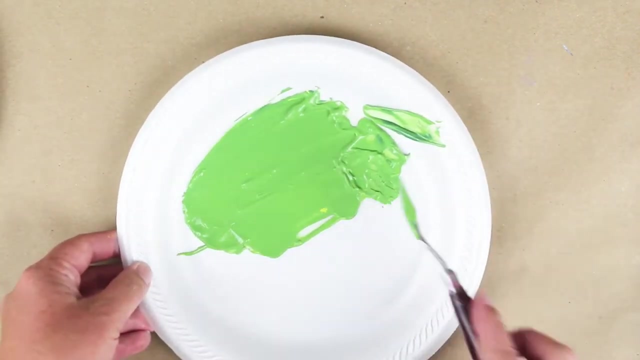 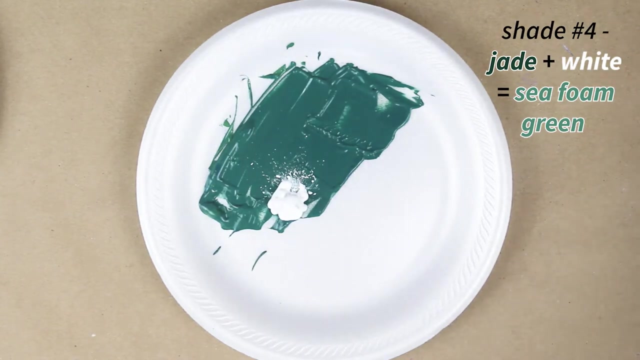 Hey everyone, I'm Sarah and this is Courageous Color, and today we'll be making 10 different shades of green. Feel free to watch them all or check the description for the time stamp of each color. I'll see you in the next video. 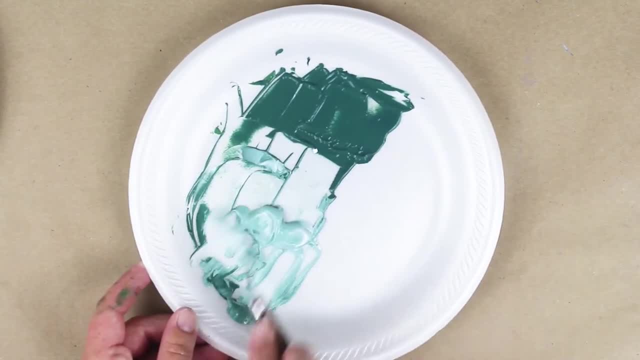 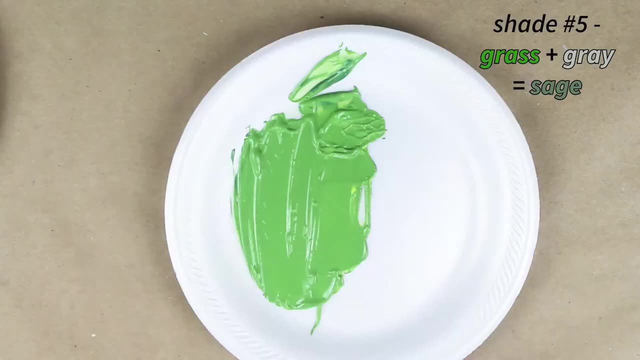 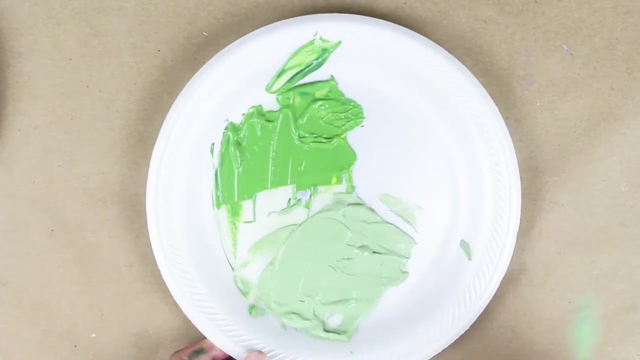 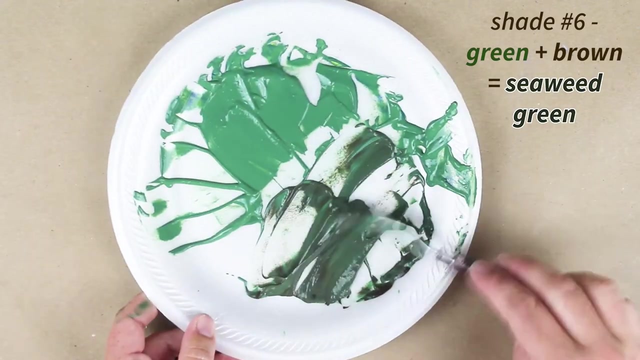 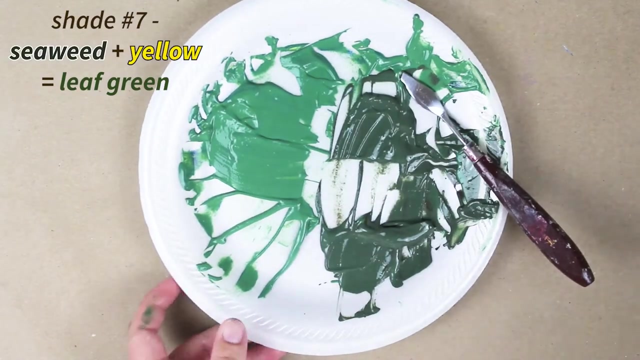 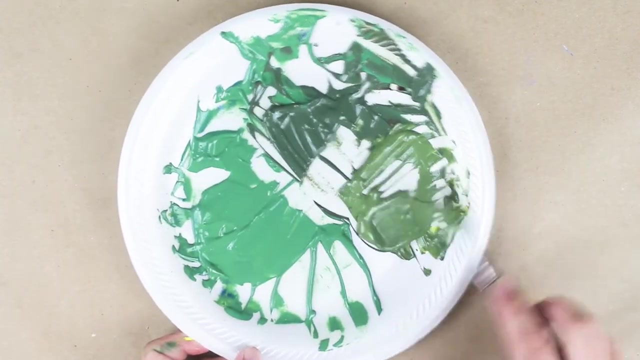 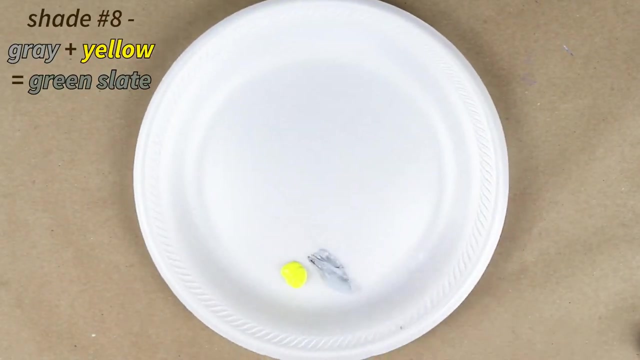 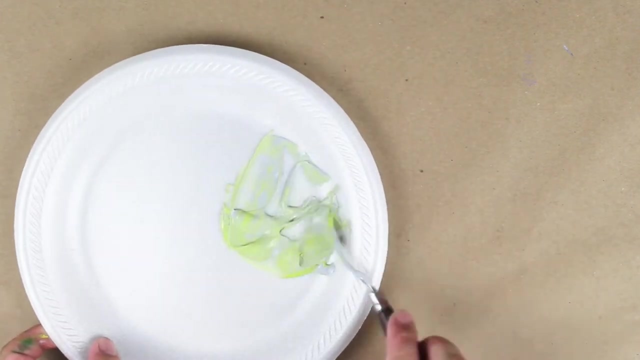 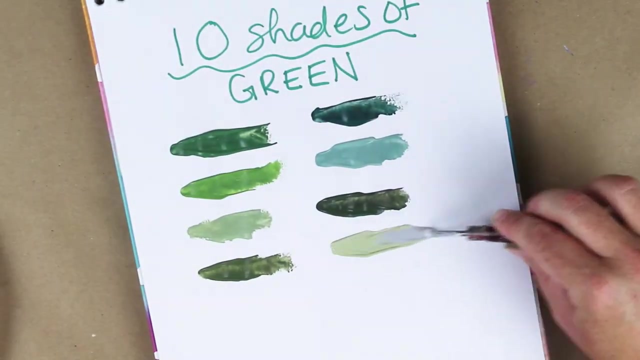 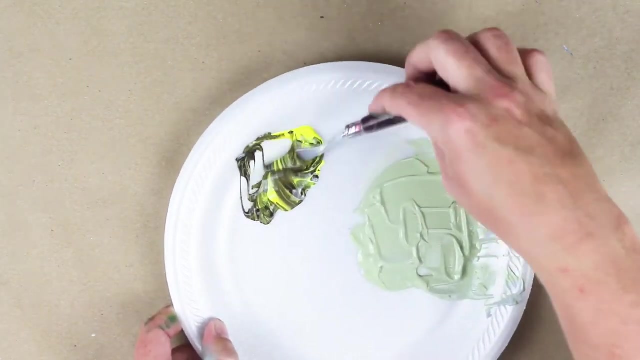 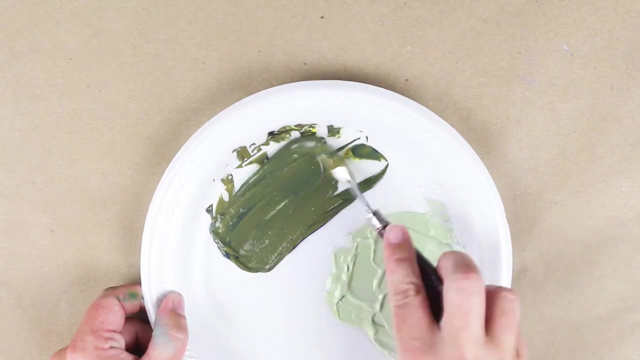 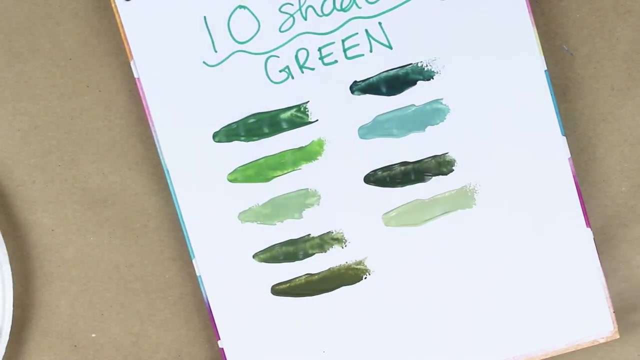 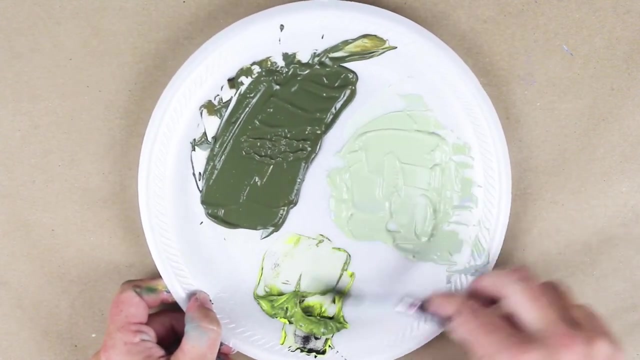 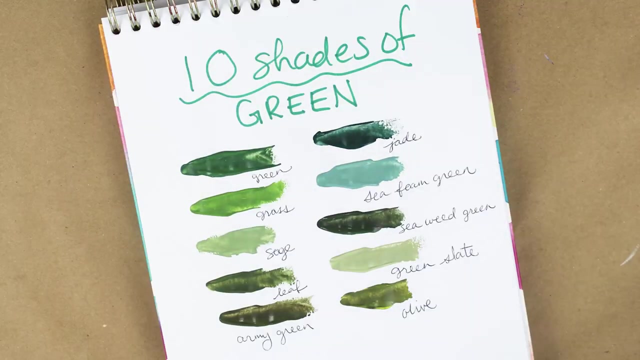 Thank you for watching. See you in the next video. Thank you for watching. See you in the next video.